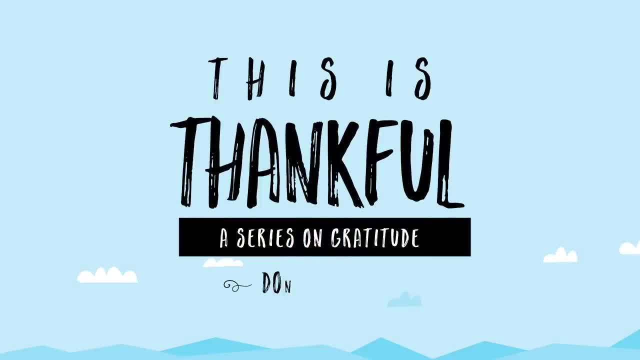 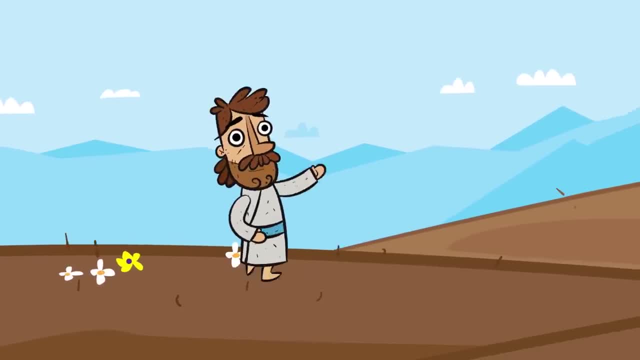 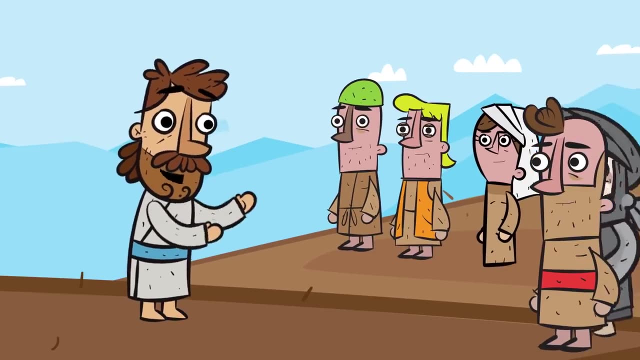 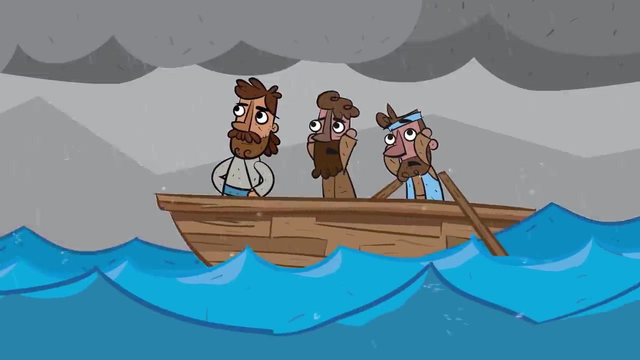 This is thankful. Don't worry, This is Jesus, who is the Son of God and the Savior of the world. Jesus did many amazing things: He taught everyone about God's love, healed people from their sickness and even calmed storms. 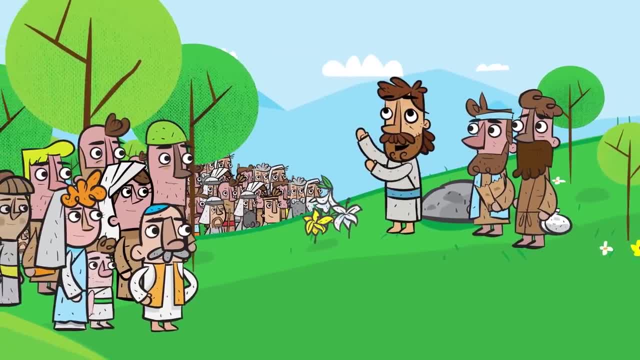 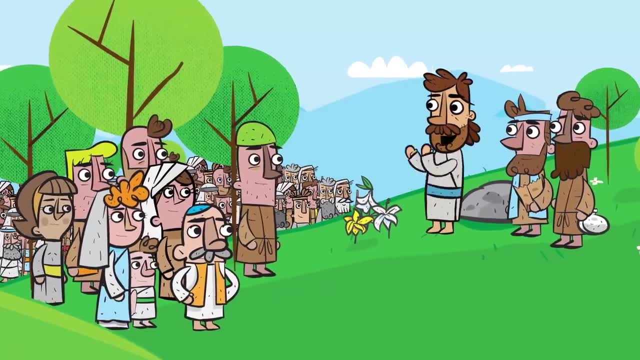 One day, Jesus was speaking to thousands of people. Hey, Jesus, When someone asked him about money, he told them a story and tried to explain to the people that our treasure is not on earth but in heaven. Then he turned to one of his disciples and said: 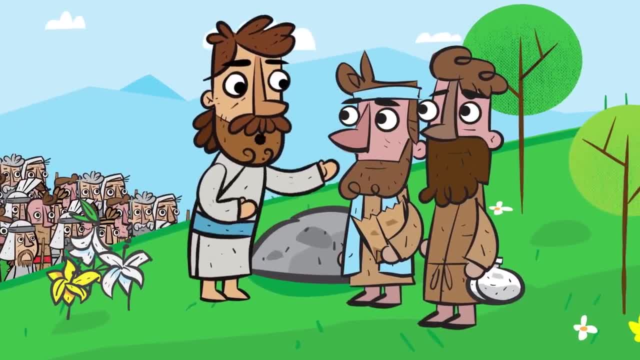 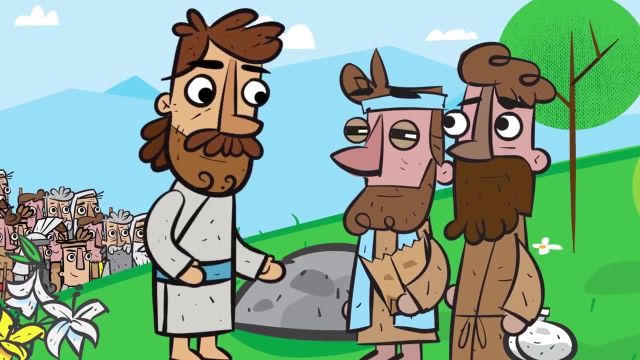 That is why I tell you not to worry about everyday life, whether you have enough food to eat or enough clothes to wear, for life is more than food and your body more than clothing. Uh yes, Look at the ravens. They don't plant or harvest or store food in barns. 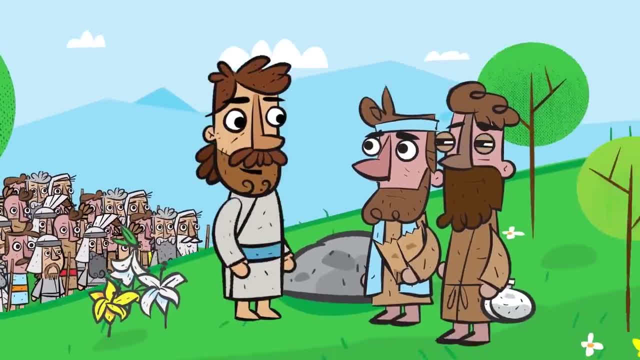 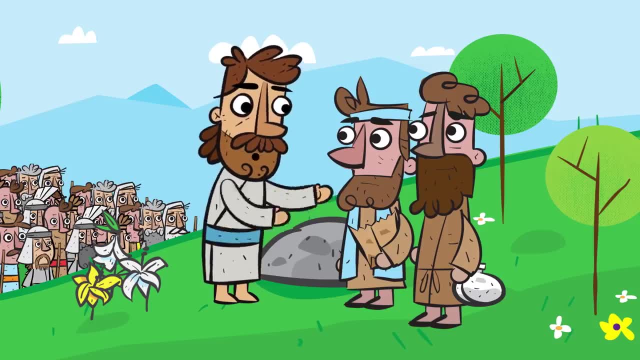 because God feeds them And you are far more valuable to God than any birds. Yeah, I think so. Do you think that by worrying about anything you can add a single moment to your life? And if worry can't do a little thing like that? 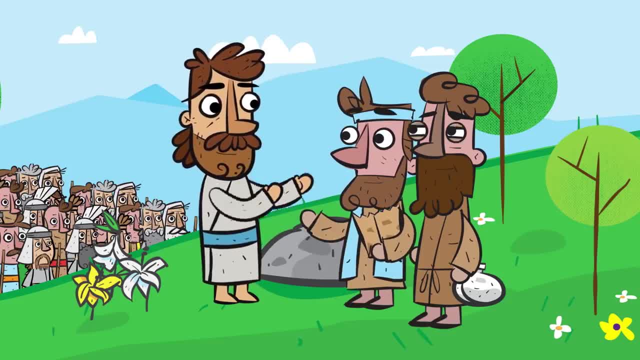 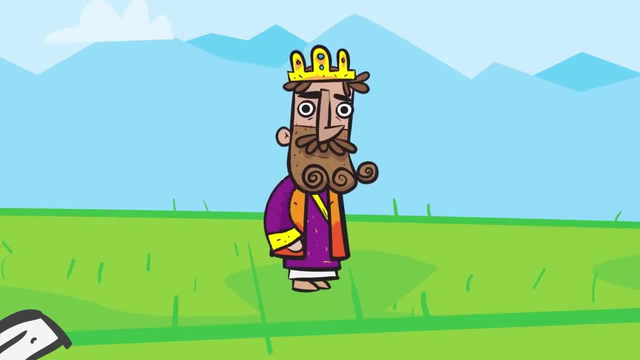 what's the use of worrying over bigger things? That's a good point. Look at all the lilies and how they grow. They don't work or make their clothing. Yet Solomon, the great king of Israel, in all his glory, was not dressed as beautifully as they are. 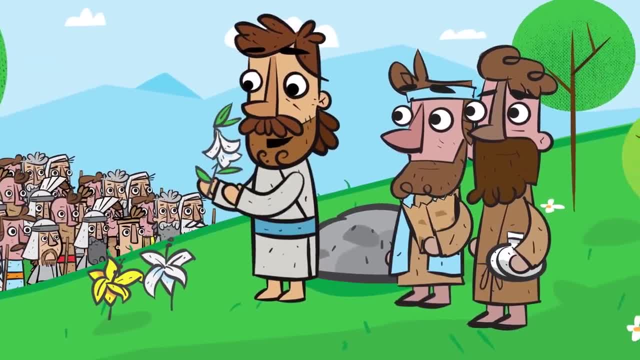 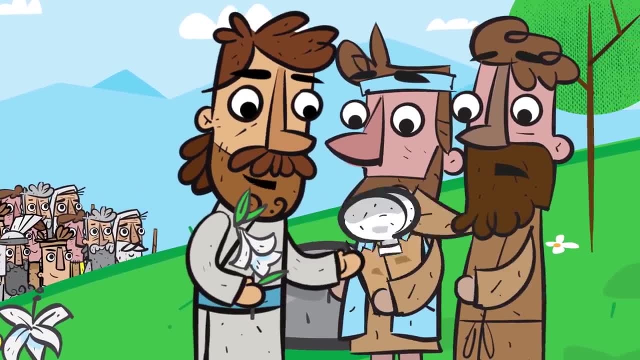 And if God cares so wonderfully for flowers that are here today and thrown away tomorrow, he will certainly care for you. And don't worry about what to eat or what to drink. Okay, Many people worry about these things, but God already knows what you need. 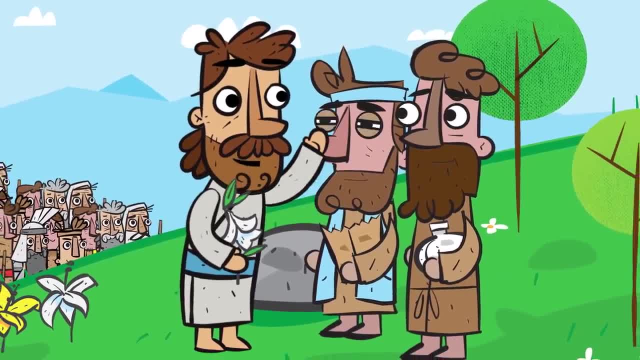 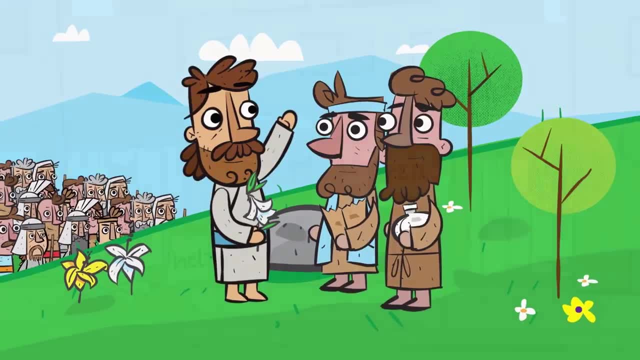 Seek the kingdom of God above all else, and he will give you everything you need. So don't be afraid, for it makes God happy to take care of you and give you his kingdom. So share what you have with others and give to those who need. 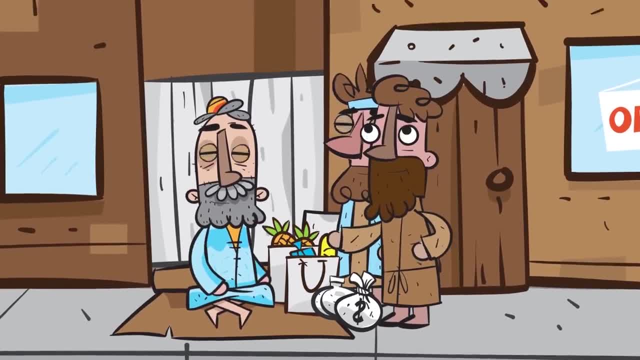 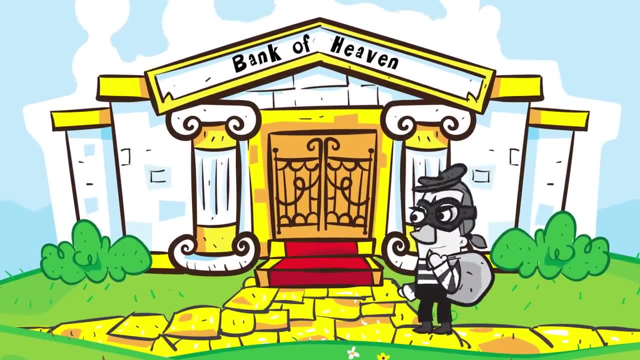 There you go. Thank you, Sure, anyhow. Then you'll be storing up treasure in heaven, And when your treasure is in heaven, it's going to be safe. No thief can steal it, Eh whatever, And no bug can destroy it.